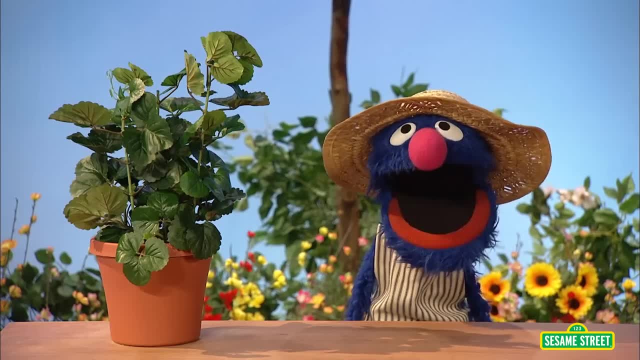 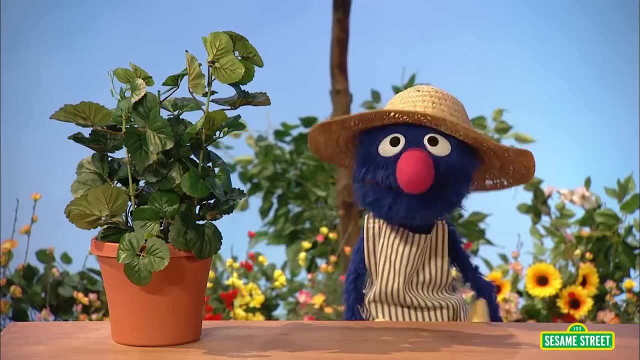 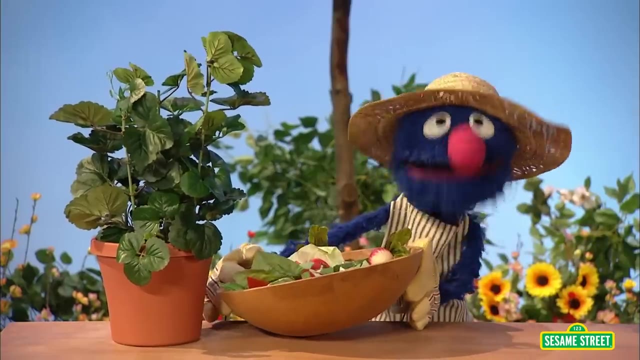 has plenty of, But a plant also needs to eat. Okay, little planty, I hope you're hungry, because oh have I got a treat for you, Something that all little plants love, and that is a big, healthful salad with radishes and tomatoes, oh and just a hint of oregano. Bon appetit. 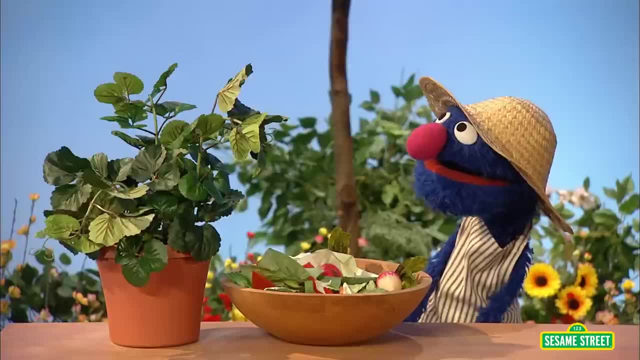 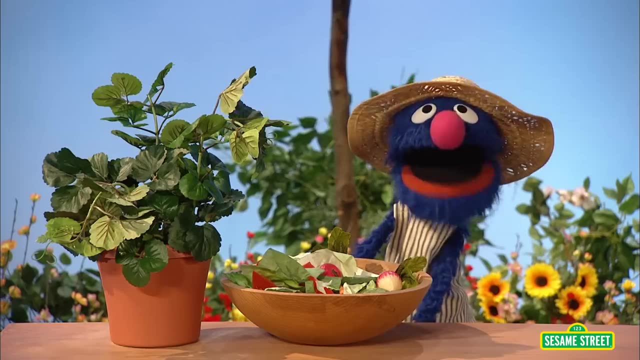 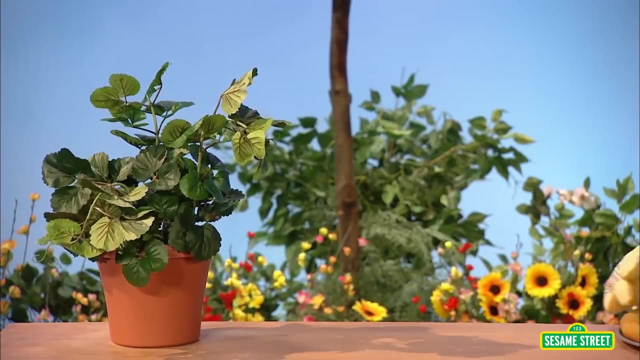 Do not wait for me, I have already eaten. Um, it appears. uh, this plant is not of the salad eating variety, But fear not, I know what else a little plant needs To grow big and healthy. A pizza, Oh oh. piping hot, fresh out of the oven. 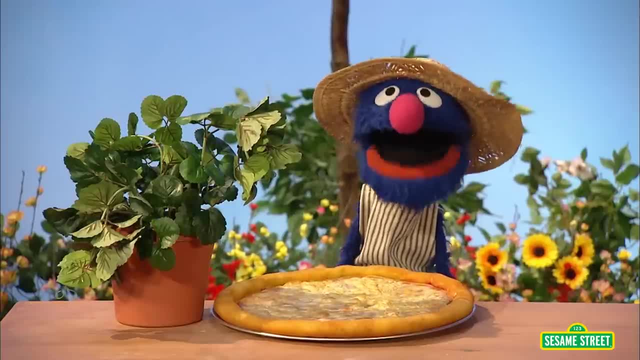 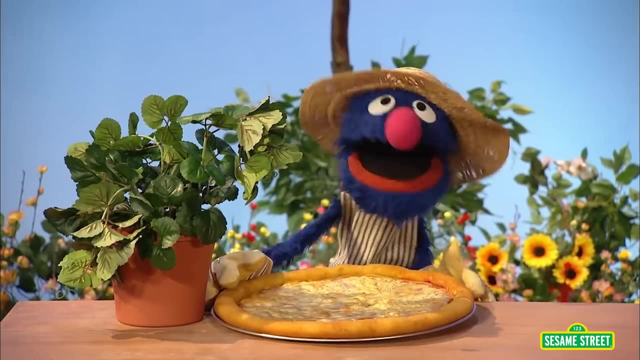 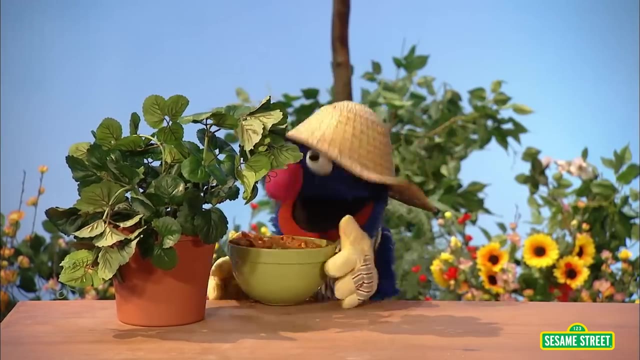 Oh dear, this little plant does not seem to be a pizza eater either, But being the resourceful gardening monster that I am, I know just the thing: that no little plant can resist Hungarian goulash. Oh enjoy, Do not resist. Give in to temptation. 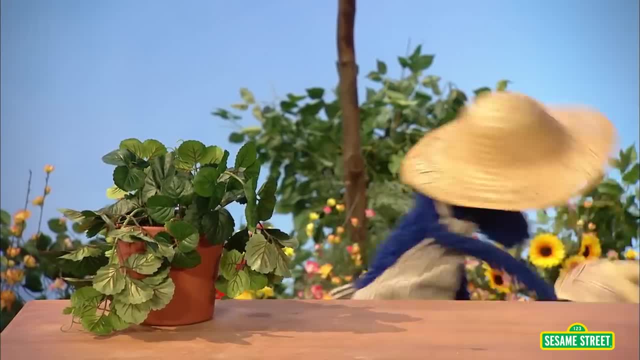 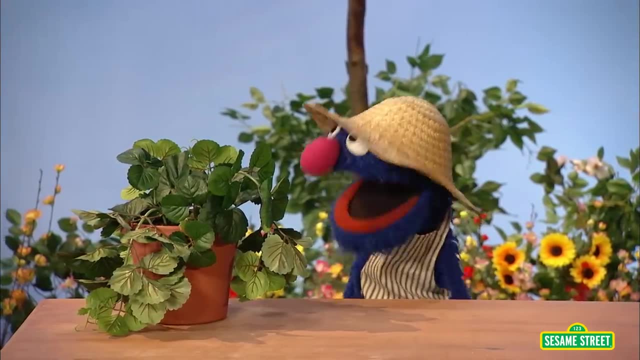 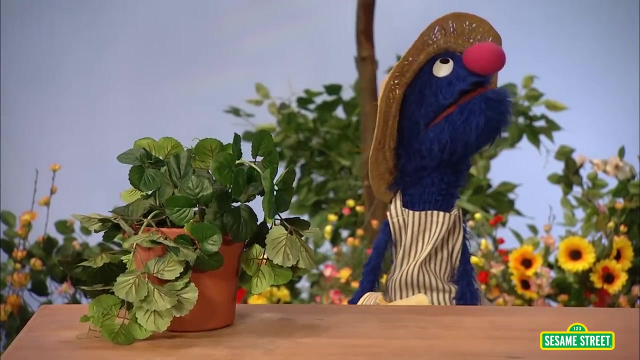 Or not, Like a vault? I cannot believe. this little plant is one finicky eater. And how will it ever grow to be big and healthy and green? and and now it is raining. Oh, the weather report did not forecast rain today, But look. 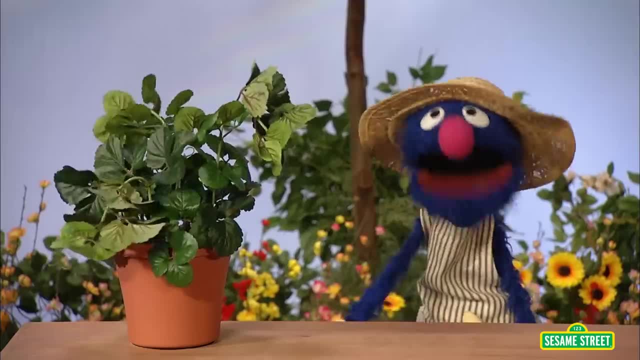 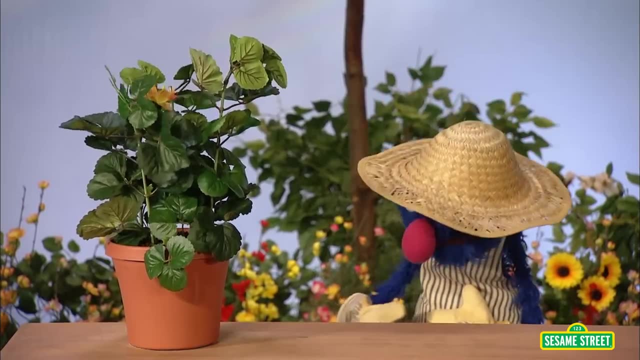 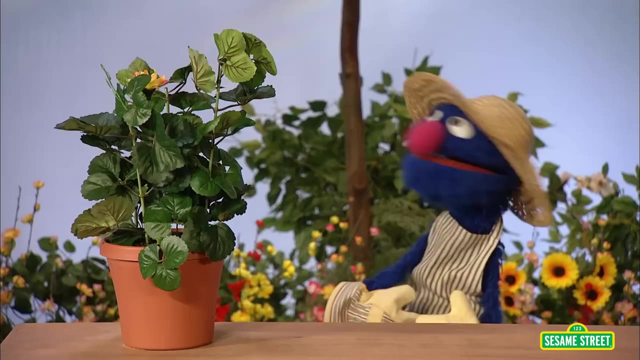 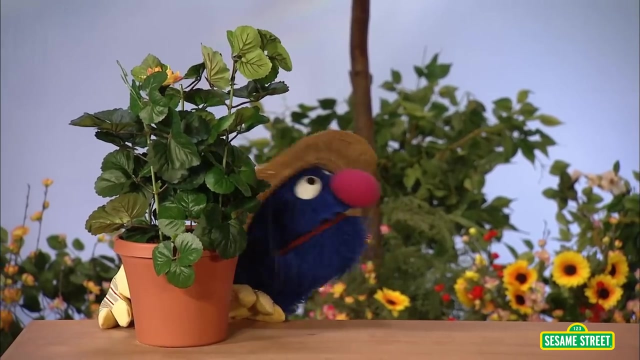 Oh, The little plant is looking nice and healthy again. Ah, I guess all it needed was a little water, And I guess what I really need right now is an umbrella. Oh, excuse me if you mind. You heard the story of the three bears. 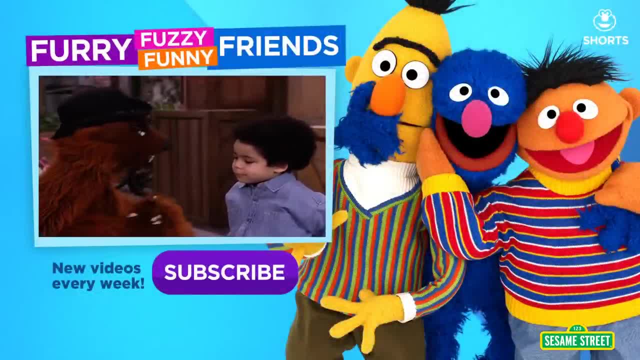 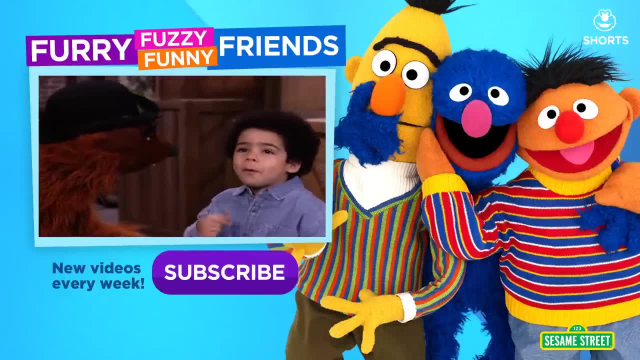 Mm-hmm. Well, that's where I live. I have three of everything: One for me, One for mama bear And one for baby bear, Just like um the story when the papa bear and the mama bear and the baby bear. 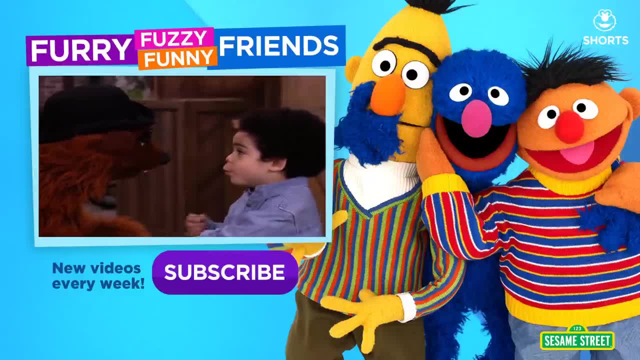 had um oatmeal and then they left it to warm up.